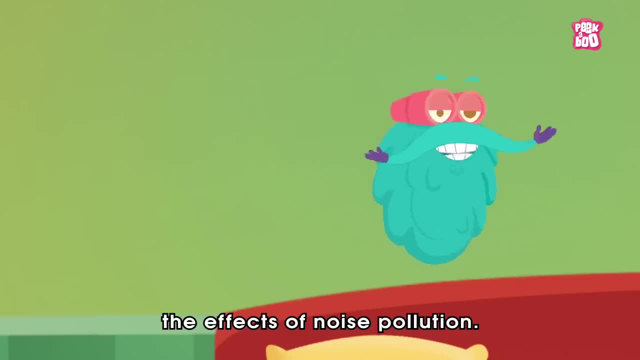 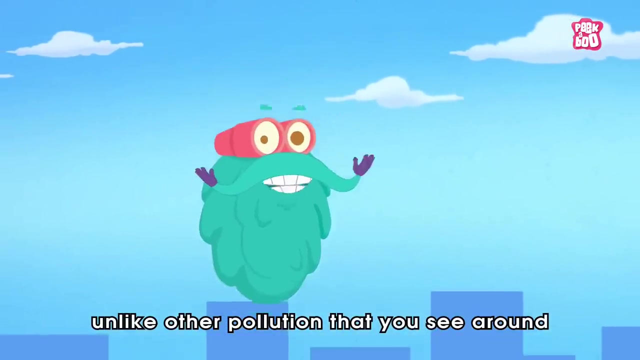 By experiencing the effects of noise pollution. Yes, my friends, in today's episode, let us explore the noisy world of noise pollution And know about its causes, effects and ways to reduce it. Zoom in, Hey, friends. unlike other pollution that you see around, like water, land, air, etc. 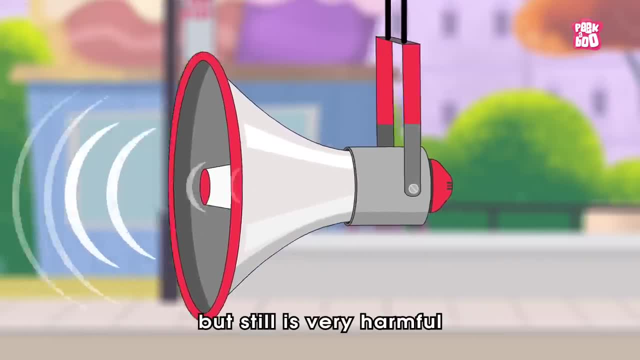 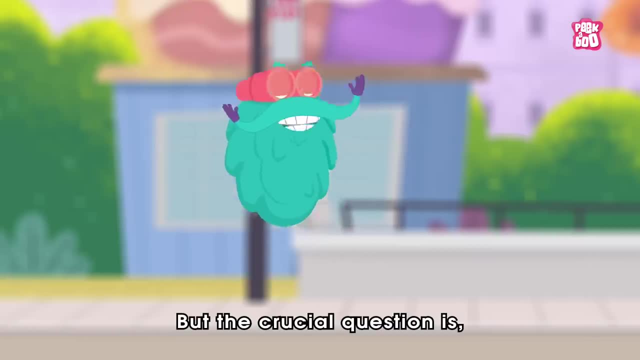 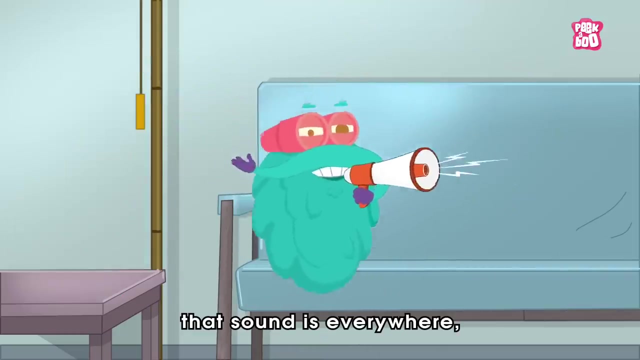 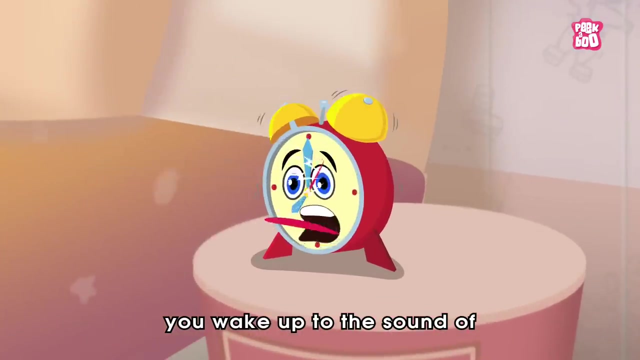 Noise pollution is invisible to you, but still is very harmful to those who get in its path. But the crucial question is: what is this noise pollution? Well, as we know that sound is everywhere, Right from the alarm clock, you wake up to the sound of, to the school bus, the school bell, loudspeakers. 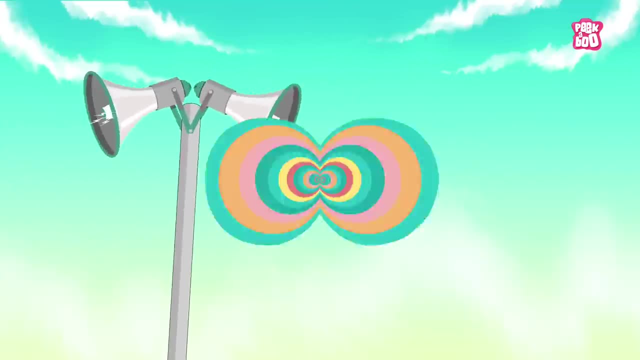 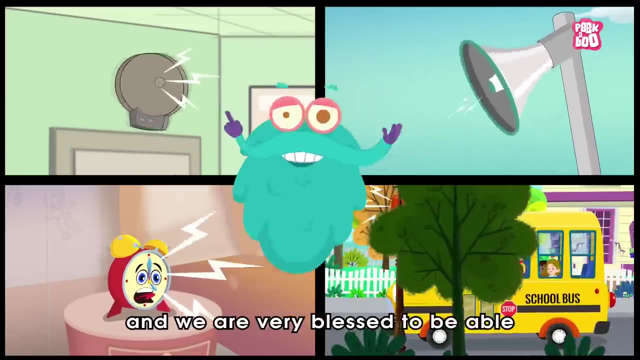 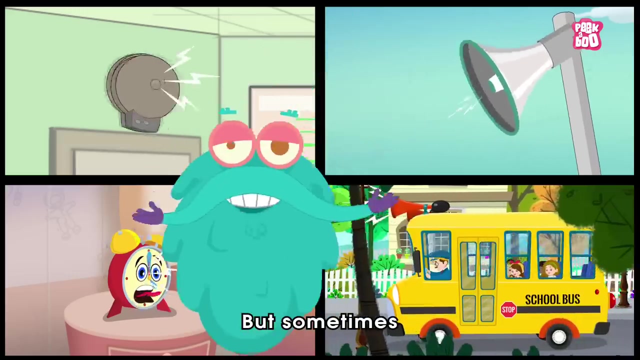 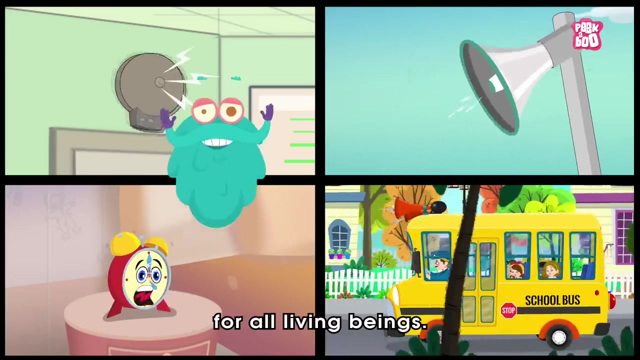 and so on, And, as we know, these sounds are a vital part of our daily routine And we are very blessed to be able to hear everything around us, But sometimes these necessary sounds reach a volume that is dangerous for all living beings. 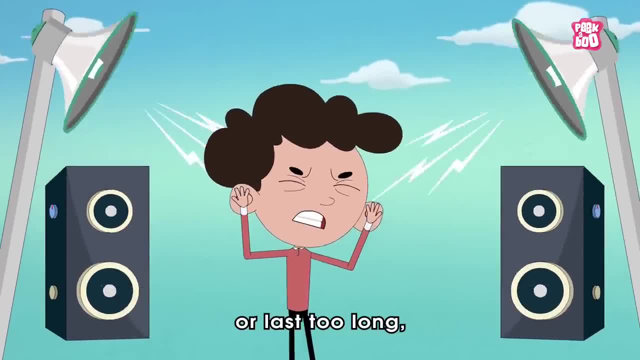 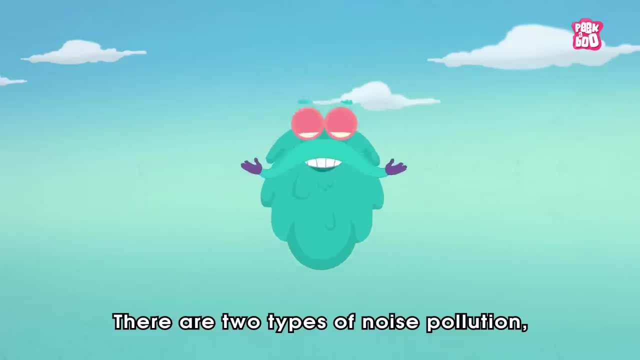 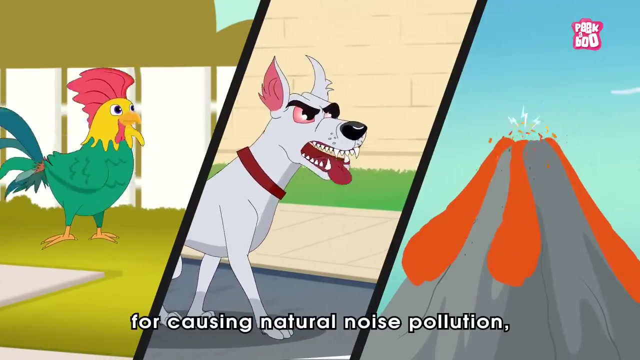 And if they get too loud or last too long, they become noise pollution. There are two types of noise pollution: natural and man-made. The sound coming from natural sources such as birds, animals and all natural calamities are responsible for causing natural noise pollution, which, most of the time, are minimal. 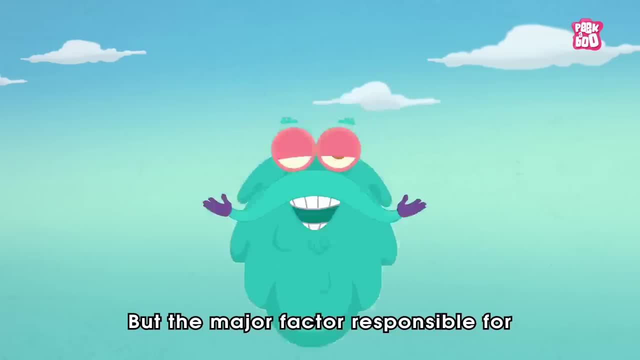 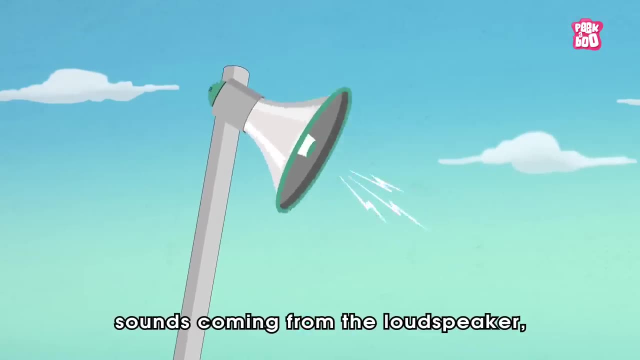 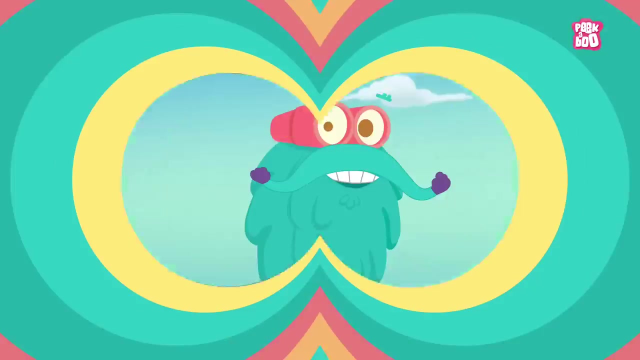 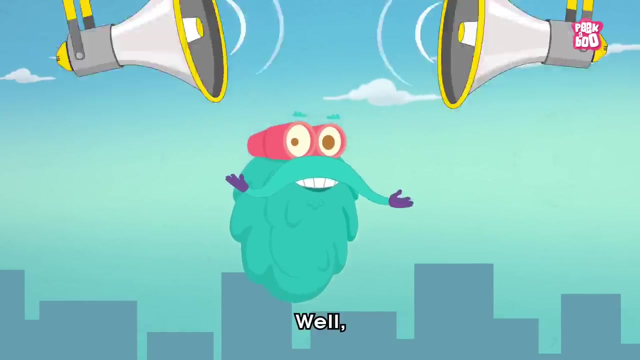 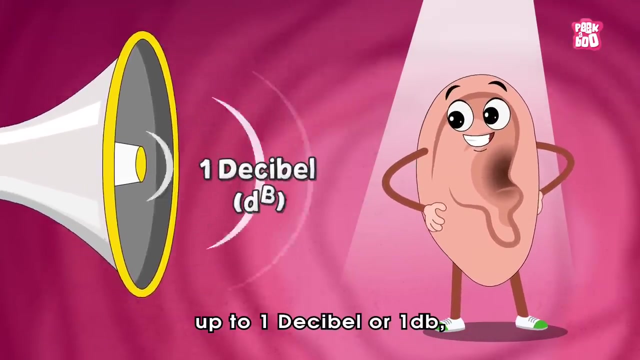 But the major factor responsible for causing noise pollution is man-made machines, Such as sounds coming from the loudspeaker, construction sites, traffic, etc. But the most crucial question is: how does sound affect our health? Well, human ears are designed to hear sound up to 1 decibel or 1 dB. 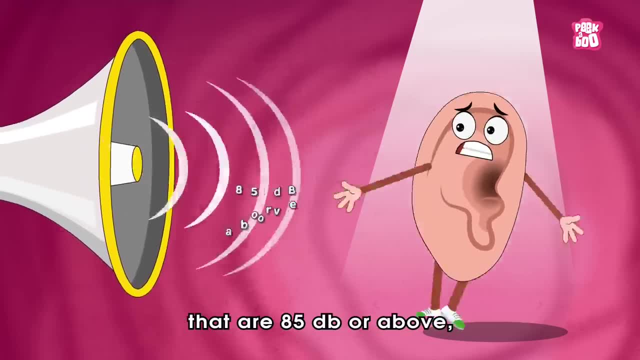 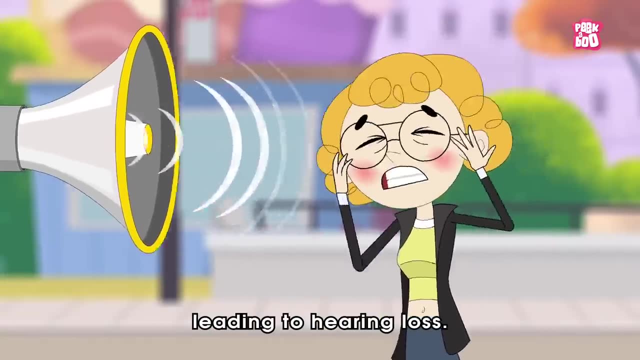 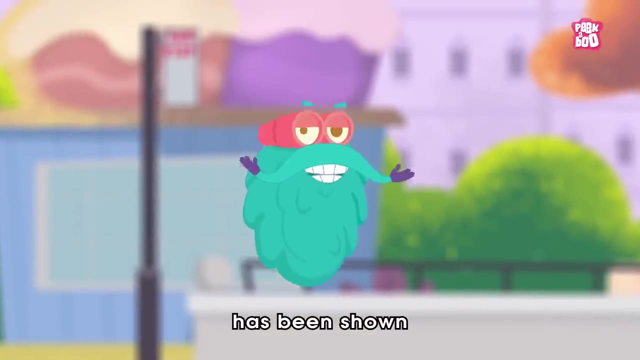 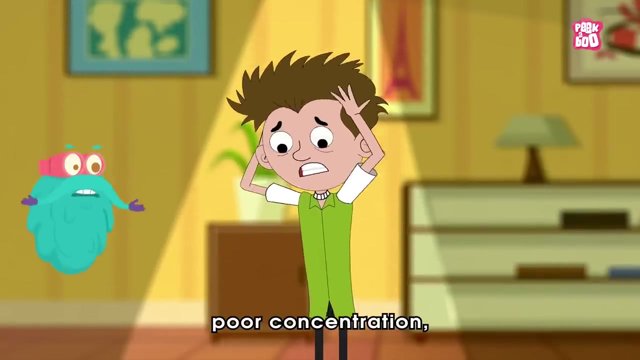 When someone is exposed to sounds that are 85 dB or above, it can cause permanent damage to your ears, leading to hearing loss. Not only that, exposure to prolonged or extreme noise has been shown to cause a range of health problems ranging from stress, poor concentration, productivity loss at work and at school. 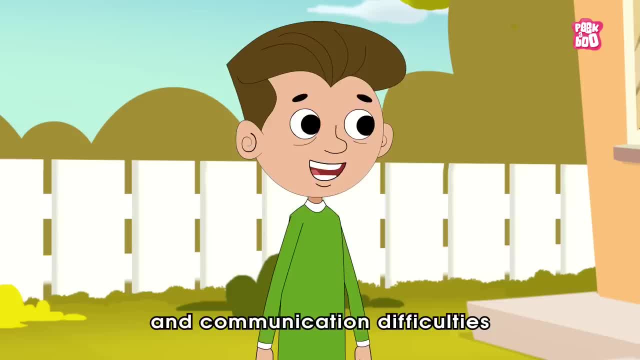 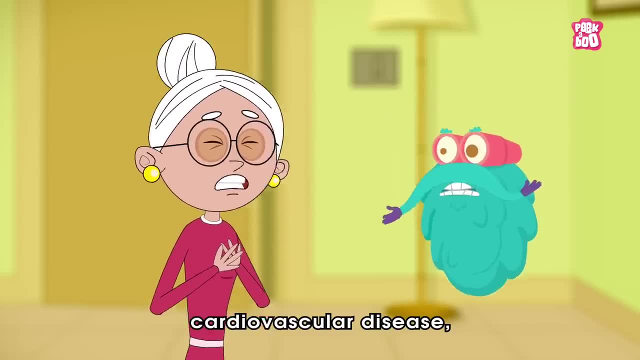 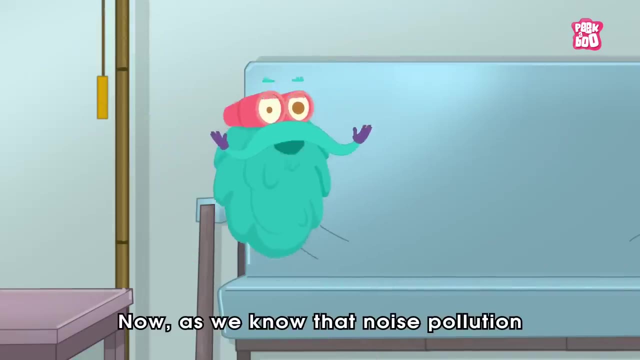 Fatigue, from lack of sleep and communication difficulties to more severe issues such as cardiovascular disease, cognitive impairment, etc. Now, as we know that noise pollution can be so dangerous, we must definitely take steps to reduce it for the betterment of our health and environment. 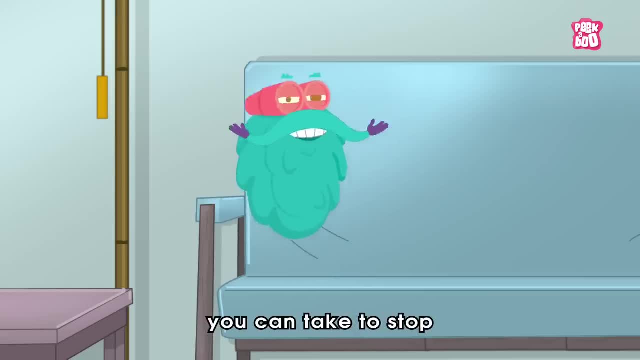 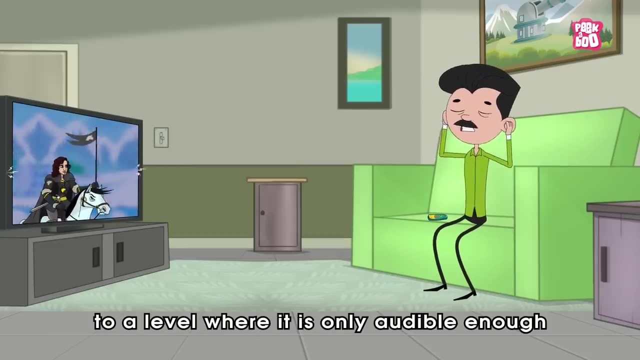 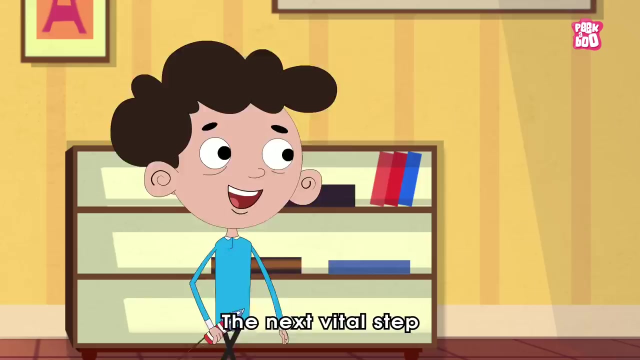 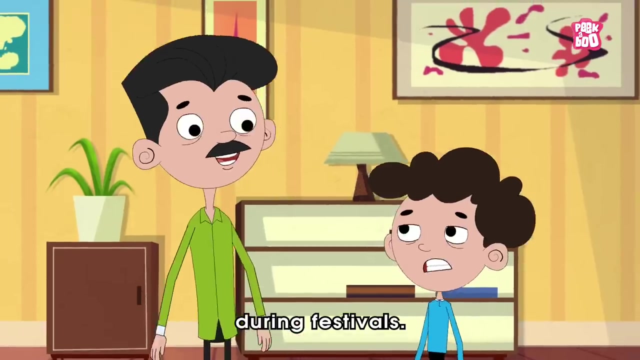 So what are the steps you can take to stop noise pollution? Well, make sure to set the volume of your TV to a level where it is only audible enough to you and not your neighbours. The next vital step is to always try to avoid noisy firecrackers during festivals. 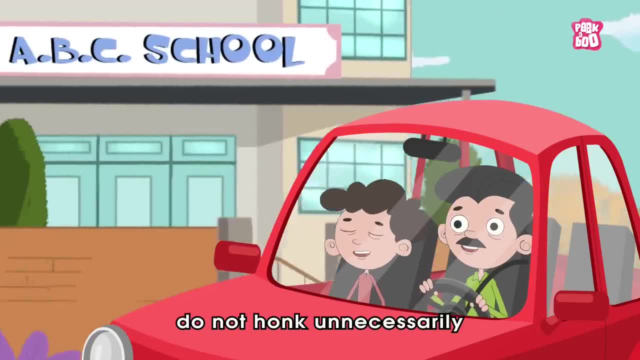 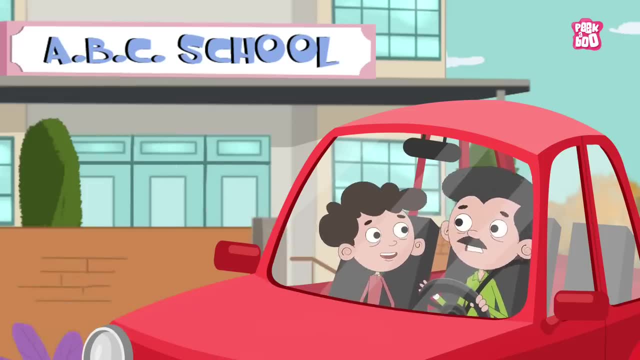 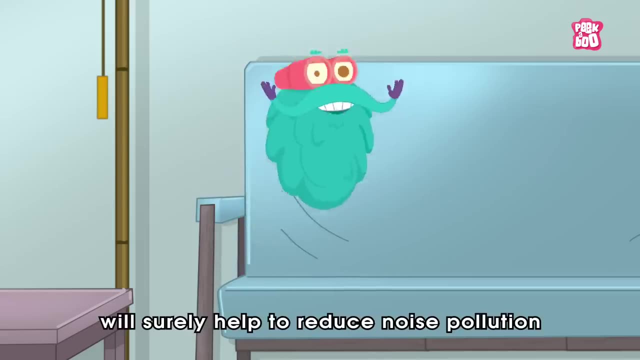 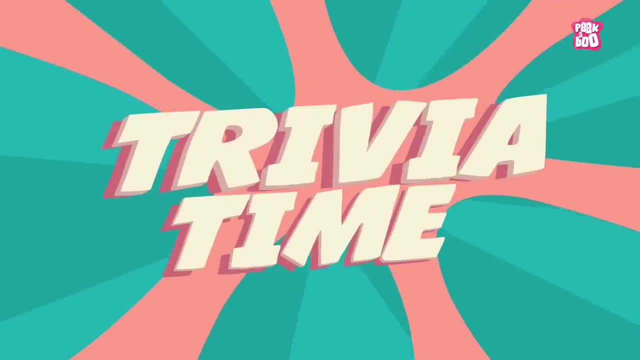 And ask your mom or dad to not honk unnecessarily and especially while passing by school or hospitals. These little steps from your end will surely help to reduce noise pollution and make our environment a peaceful place to stay in. Did you know we are not the only ones affected by noise pollution? 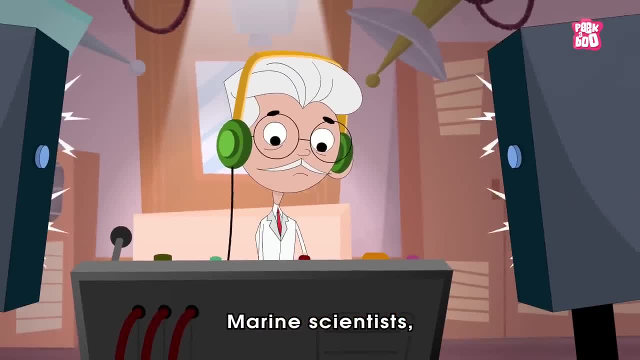 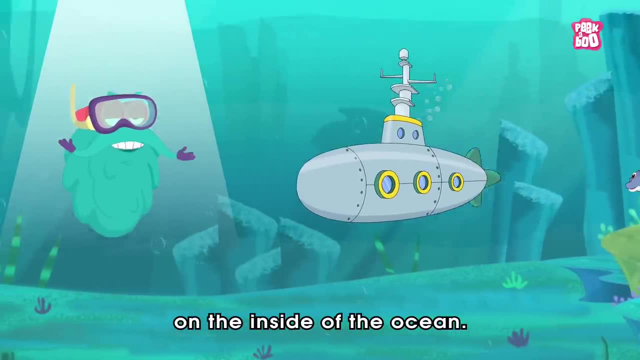 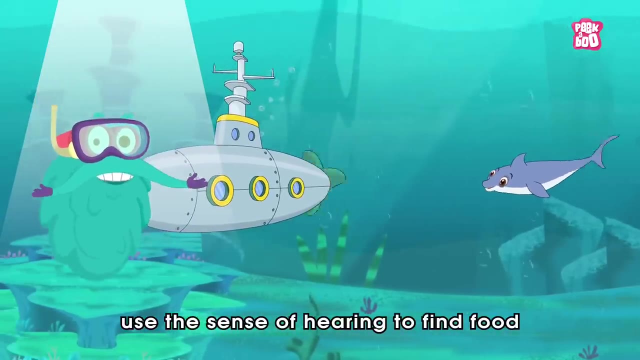 Yes, my friends, marine scientists are concerned with the excessive noise used by oil drills and submarines on the inside of the ocean, And as many aquatic animals use the sense of hearing to find food or to defend themselves to survive in the sea. 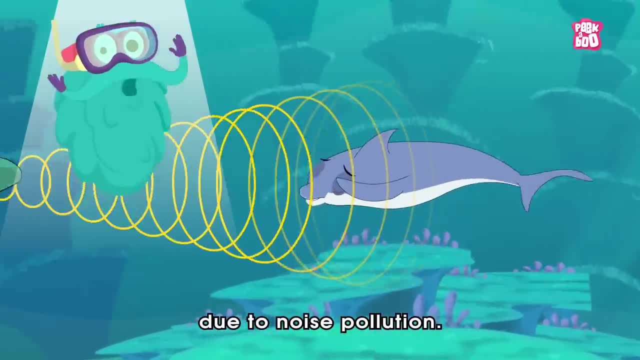 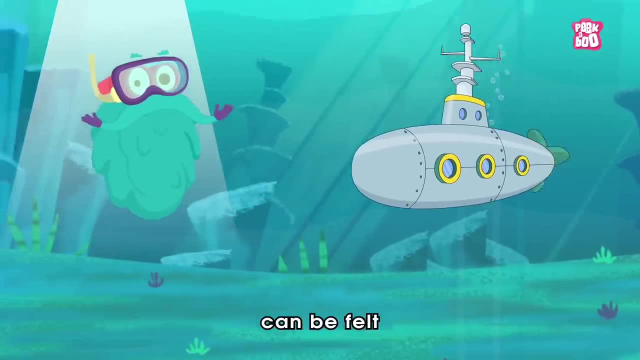 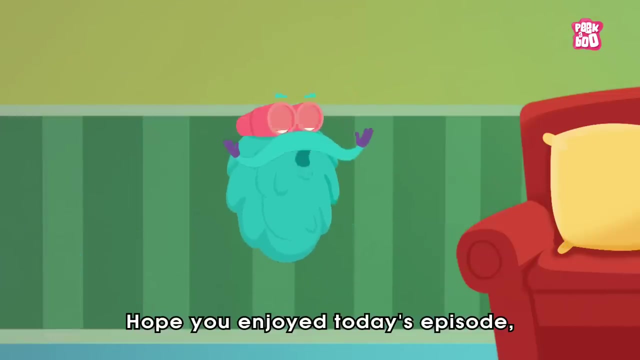 they are at a higher risk due to noise pollution. Also, you won't believe, but a submarine sonar can be felt .300 miles away from the source. Hope you enjoyed today's episode. Until next time. it's me, Dr Binox, zooming out.